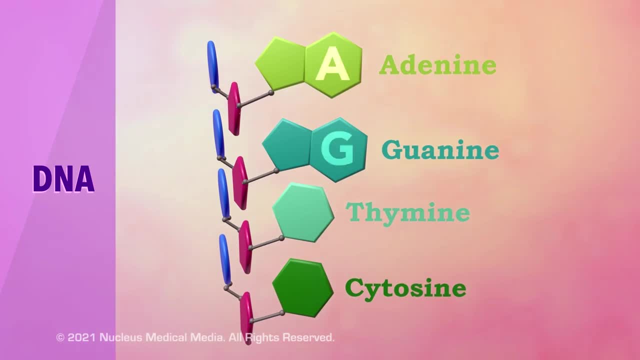 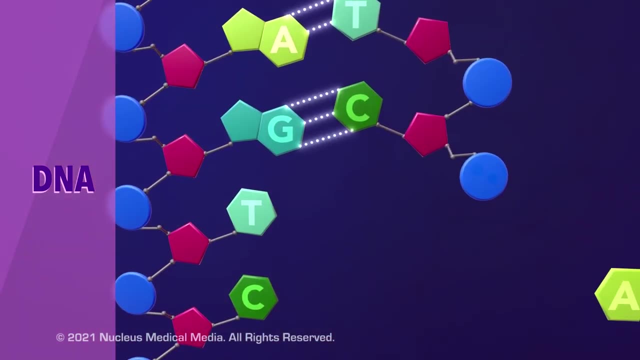 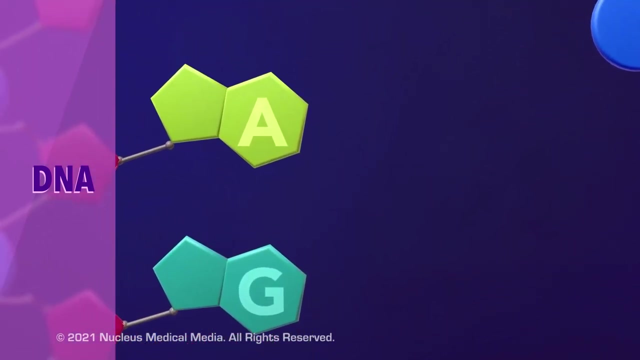 These four bases are usually abbreviated A, G, T and C. When nucleotide bases connect through hydrogen bonds, it's important to know that the bases always pair together. If the bases only pair up with the same partners, adenine only pairs with thymine and guanine. 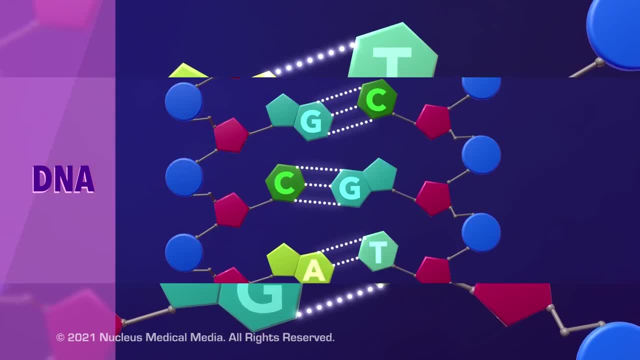 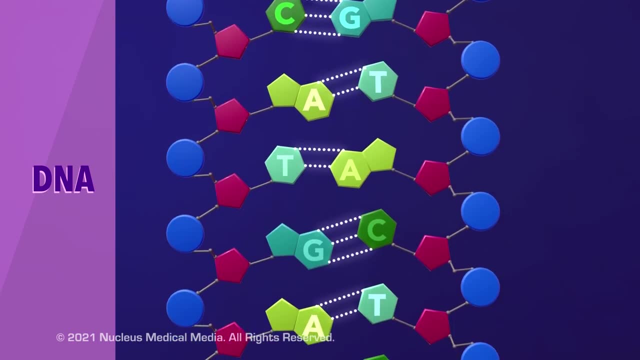 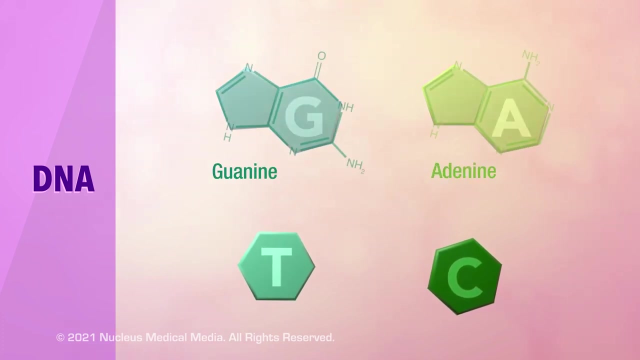 only pairs with cytosine. This is called the base pair rule. Scientists classify nitrogenous bases according to the shape of their molecules. Adenine and guanine. both have a double ring structure containing a 6-membered and a 5-membered. 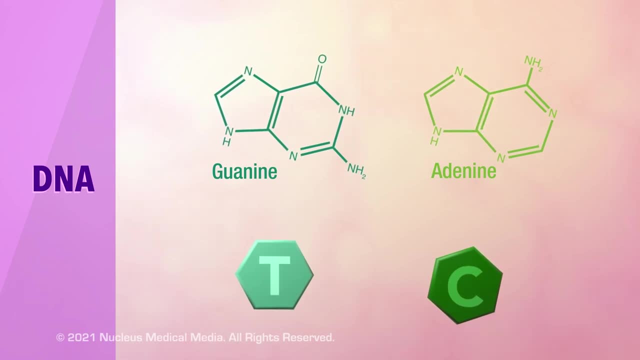 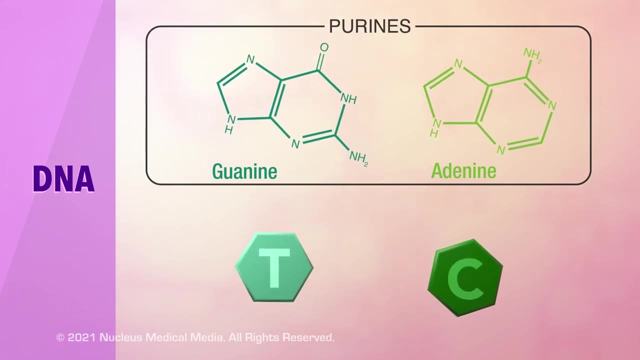 nitrogen-containing ring ring fuse together. These types of ring structures are chemically classified as purines, But thymine and cytosine both only have a single six-membered nitrogen-containing ring shape, so they are chemically classified as pyrimidines. Here's a little hint to help you remember. 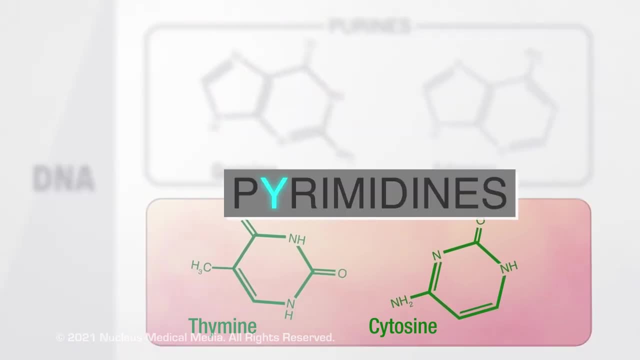 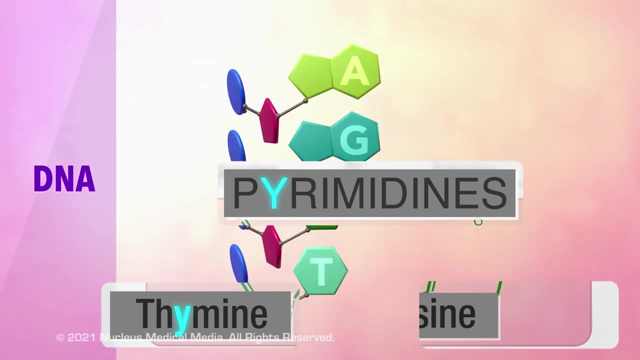 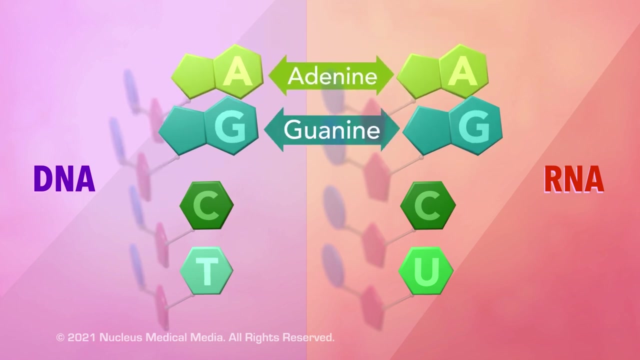 this Pyrimidine has a Y in its name, and so do the bases classified as pyrimidines, thymine and cytosine. Like DNA, an RNA nucleotide may have the nitrogenous bases adenine, guanine. 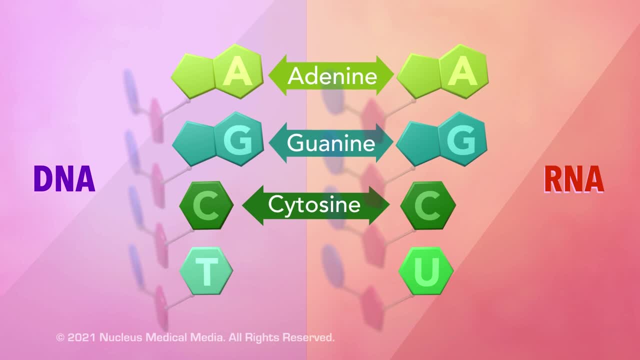 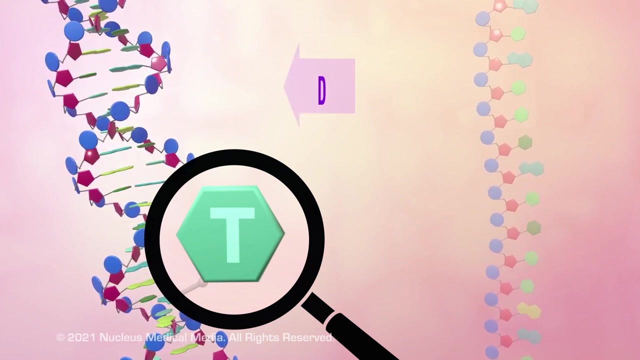 or cytosine, But unlike DNA, which has the nitrogenous base thymine, RNA has the nitrogenous base uracil instead. Thank you. This means that any nucleic acid that contains thymine must be a strand of DNA and that 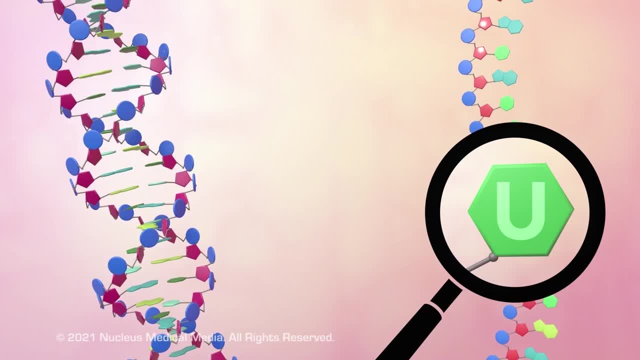 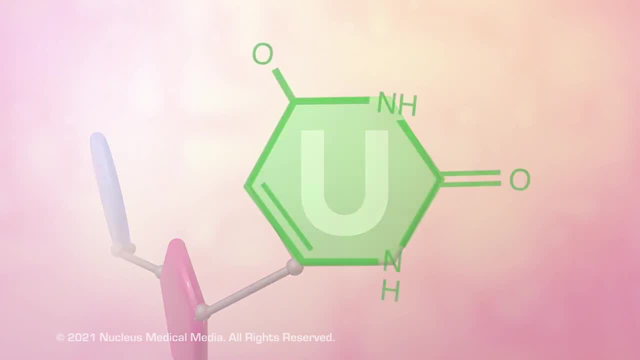 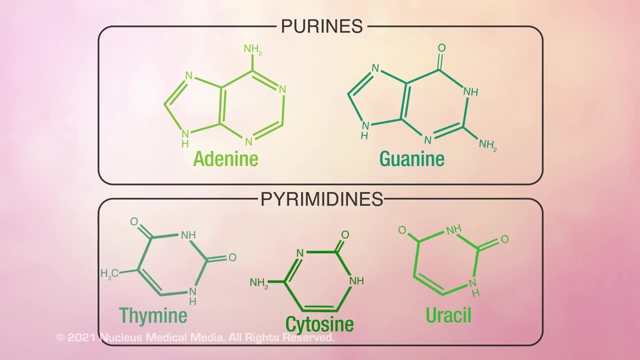 any nucleic acid that contains uracil must be a piece of RNA. Like thymine, uracil has a single nitrogen-containing ring, so it would also be classified as a pyrimidine. So what do the nitrogenous bases have to do with thymine? 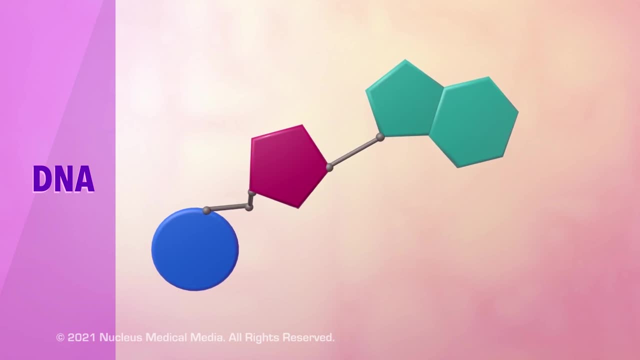 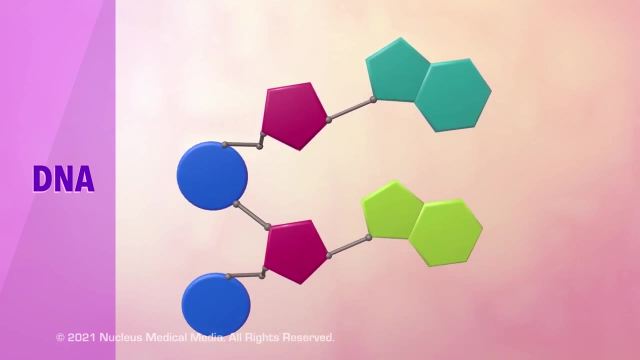 First, they have to create a molecule, which is called a DNA molecule. Well then, each strand that has a DNA molecule is important. But first, why does that DNA molecule have to do with building a DNA molecule? Well, each strand of DNA begins to assemble when the phosphate group in one nucleotide 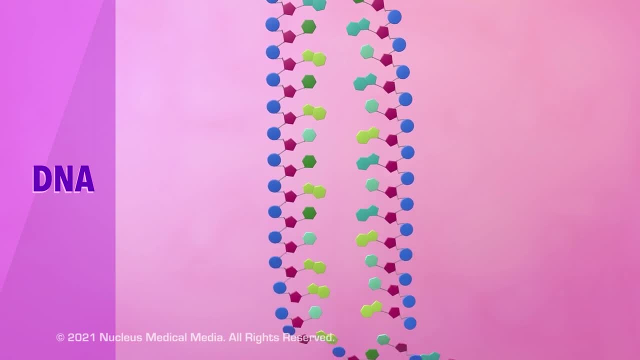 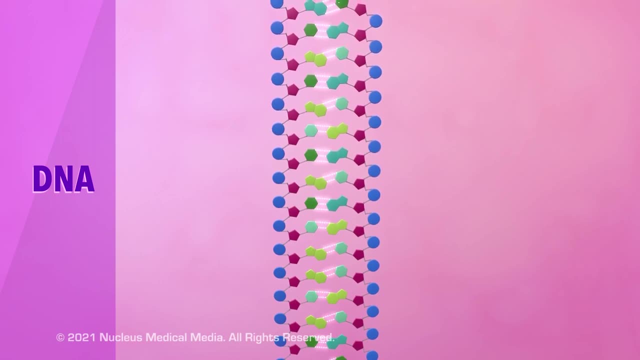 bonds with the five-carbon sugar in another nucleotide. The two strands that make up a DNA molecule are linked through hydrogen bonds between their nitrogenous bases. Now, if the example shows you how it works, here's a quick example. We've got a DNA molecule. 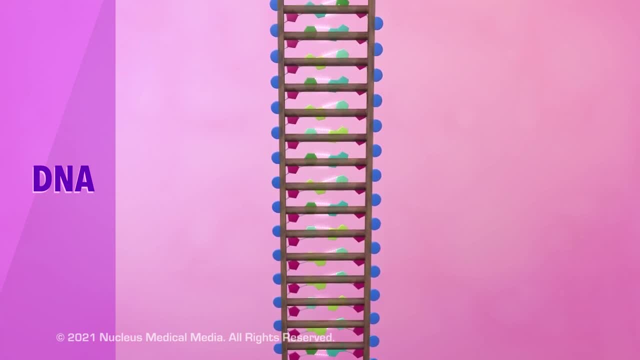 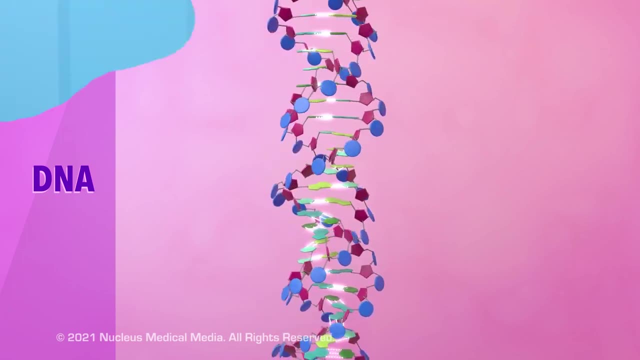 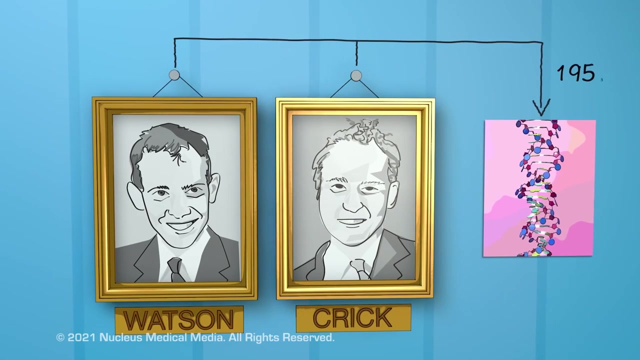 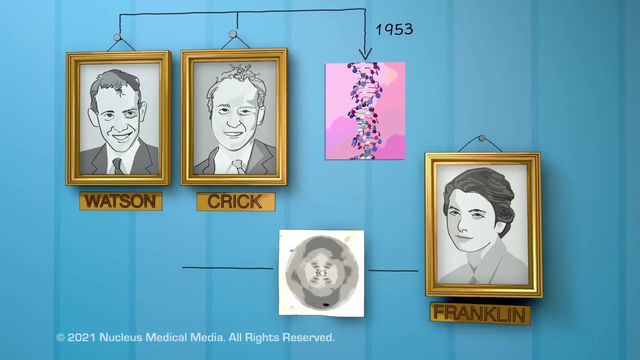 look like rungs on a ladder. The spiral DNA molecule is described as having a double helix shape. James Watson and Francis Crick first described DNA's double-stranded helical structure in 1953, after looking at X-ray images of a DNA molecule taken by Rosalind Franklin. 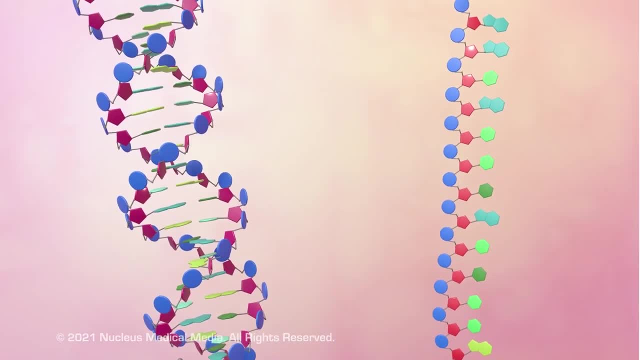 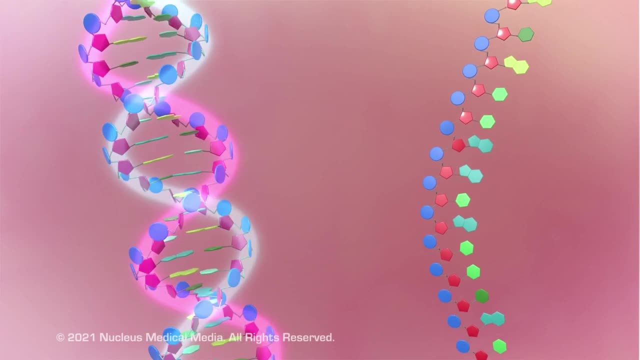 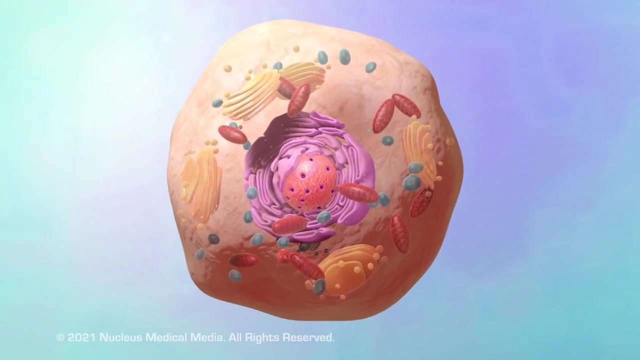 Now let's look at the structure of RNA and see how it compares to the structure of DNA. While DNA is a double-stranded molecule, RNA is always single-stranded. In eukaryotic cells, DNA is found only in the nucleus. 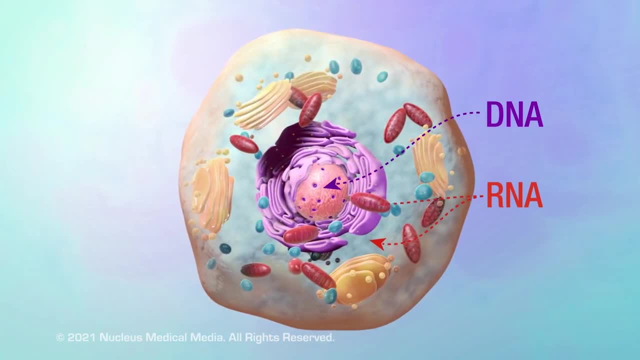 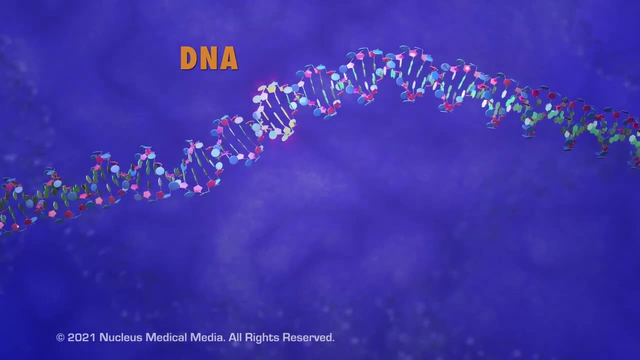 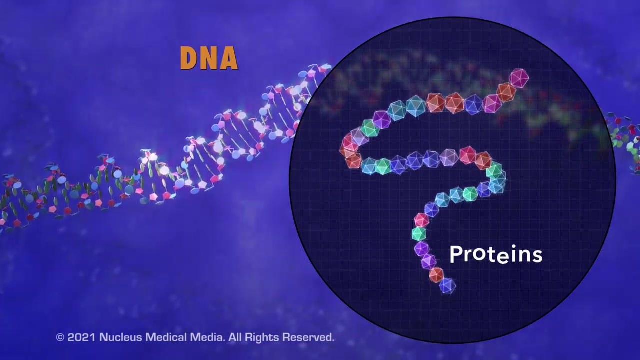 But RNA can be found in the cytoplasm as well as in the nucleus. DNA is a single-stranded molecule. RNA controls heredity by containing the code or set of instructions for building the functional and structural proteins that make up your body. 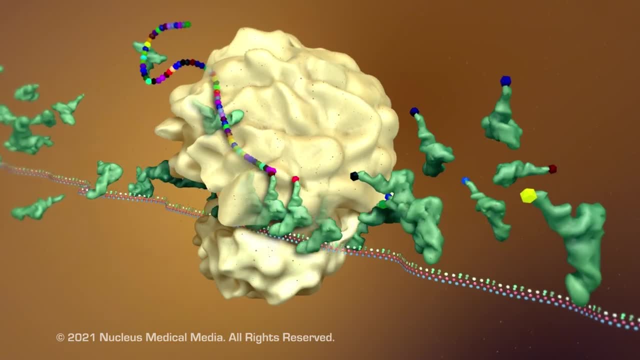 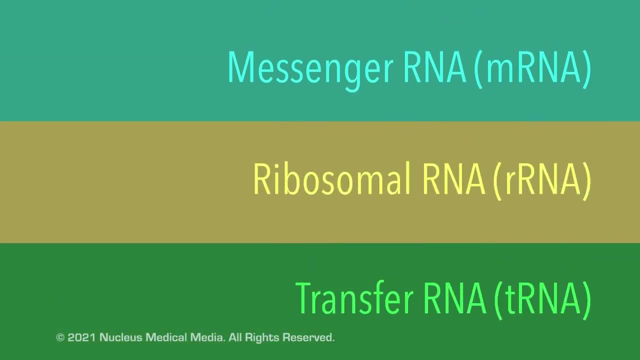 And RNA uses these varied instructions to build all the proteins a living organism needs. There are three types of RNA: Messenger RNA, referred to as mRNA, Ribosomal RNA And transfer RNA, referred to as tRNA. Messenger RNA starts off in a cell's nucleus. 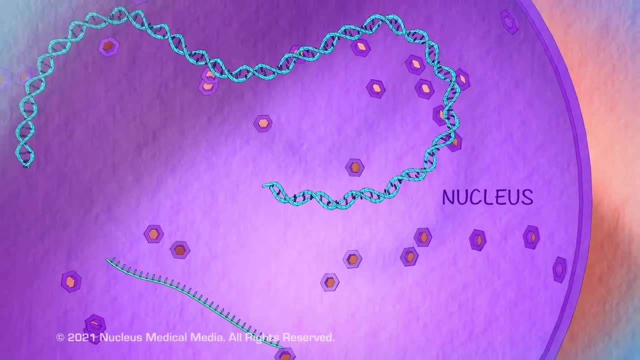 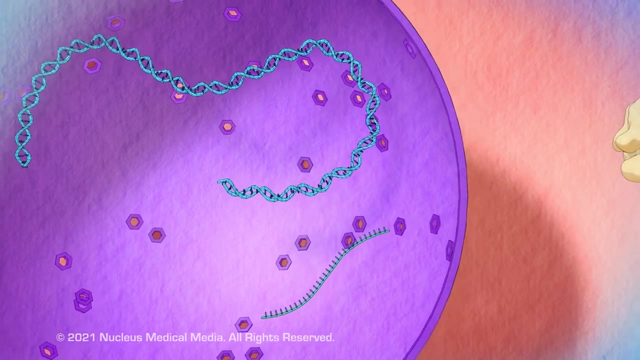 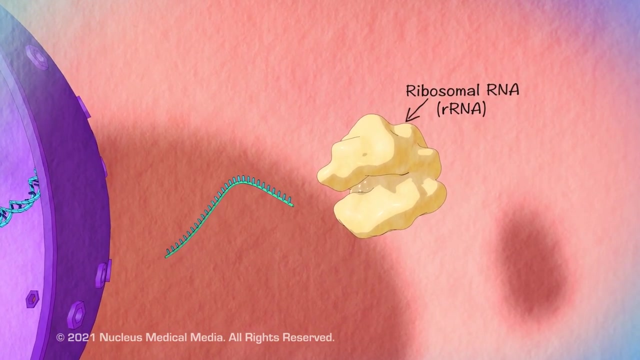 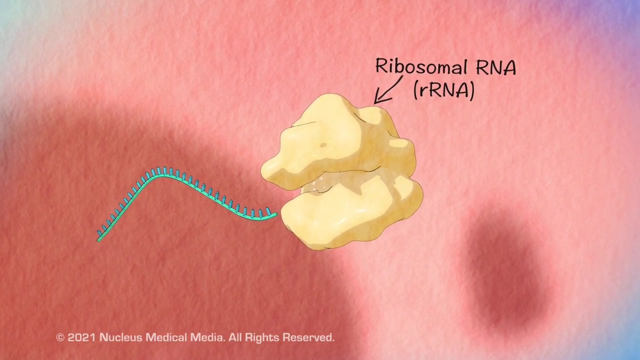 Here it transcribes or copies the instructions for assembling a protein from a portion of the cell's DNA. Next, the messenger RNA takes these instructions or protein recipe to a ribosome in the cell's DNA. The ribosome, which is made out of ribosomal RNA and proteins, is the site where this recipe. 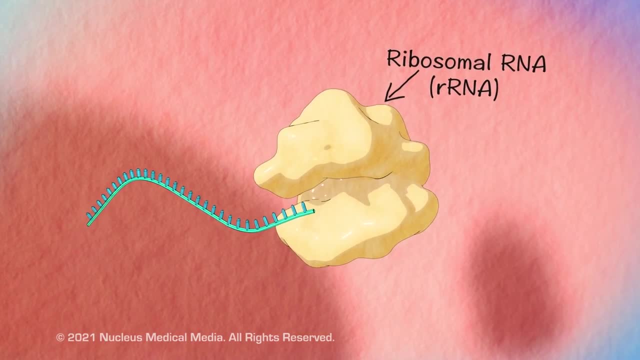 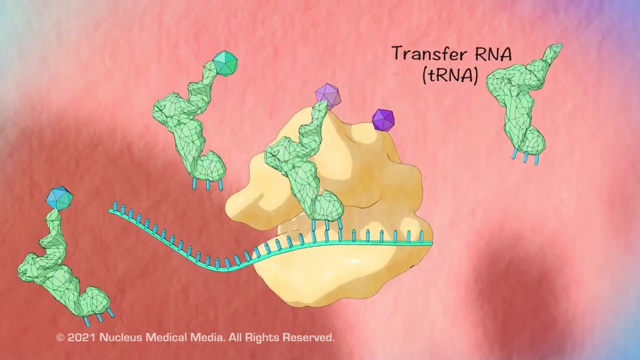 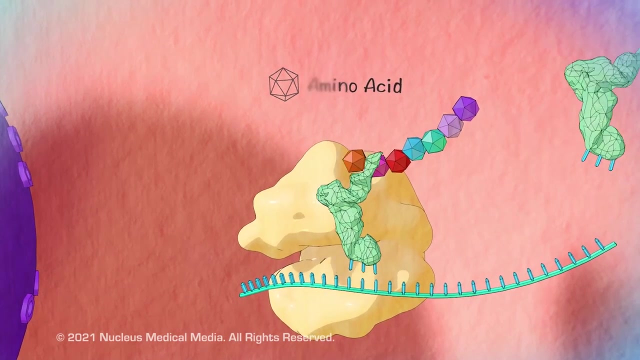 is read and translated into a protein. Finally, transfer RNA in the cytoplasm brings specific amino acids to the ribosome so that the particular protein encoded by the recipe can be made. We'll cover more deeply in a few minutes. Thank you. 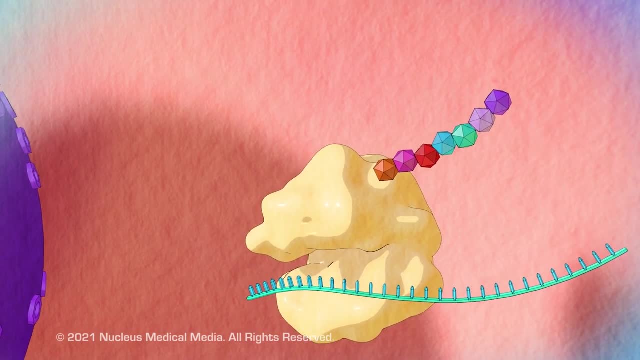 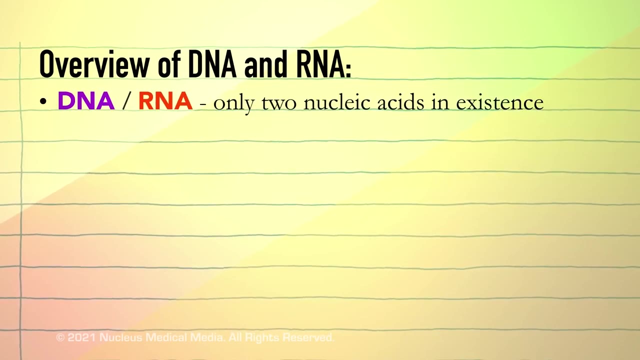 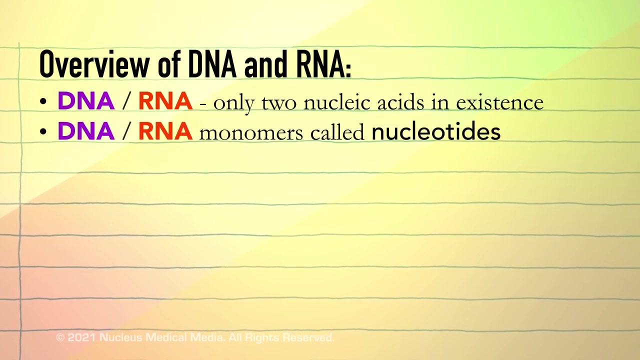 Now we'll have to get into more detail about the way DNA and RNA make proteins in another video. To sum up, DNA and RNA are the only two nucleic acids that exist. Both DNA and RNA are built from nucleic acid monomers called nucleotides. 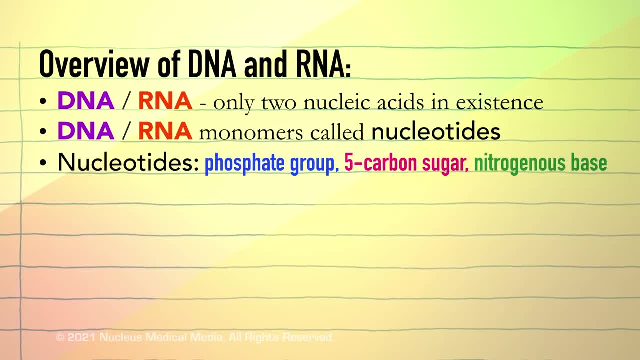 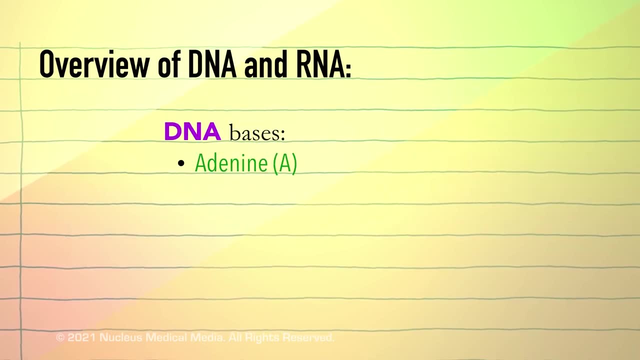 Nucleotides always contain a phosphate group, a five carbon sugar and a nitrogenous base. Deoxyribose is the sugar in between DNA and ribose is the sugar in RNA. The nitrogenous bases in DNA are adenine, thymine, cytosine and guanine. 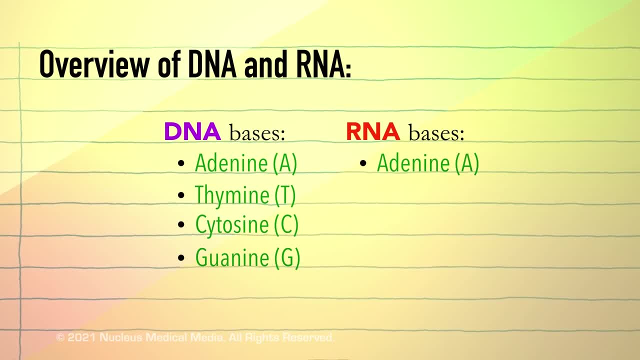 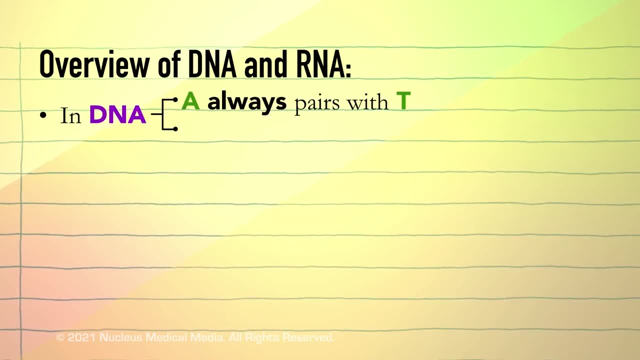 The nitrogenous bases in RNA are adenine, uracil, cytosine and guanine. In DNA, adenine always pairs together with thymine and cytosine always pairs together with guanine. Cytosine and guanine are purines. cytosine, thymine and uracil are pyrimidines. 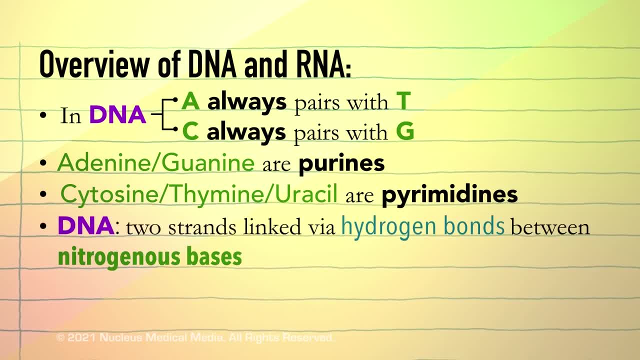 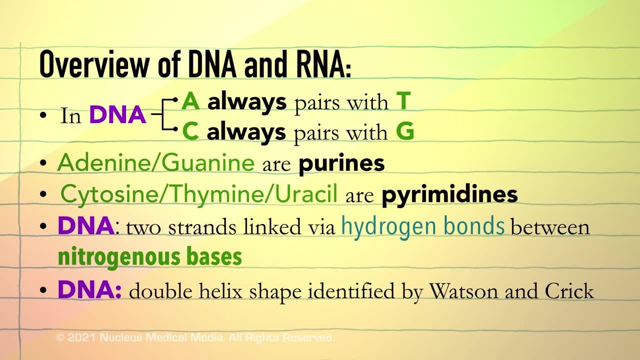 DNA is composed of two strands linked through hydrogen bonds between their nitrogenous bases. The two DNA strands are twisted into a double helix shape first identified by Watson and Crick. RNA is a single-stranded molecule. In cells, DNA is found only in the nucleus, while RNA is found only in the nucleus. 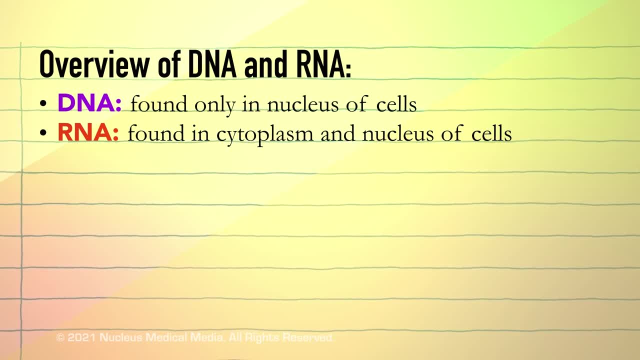 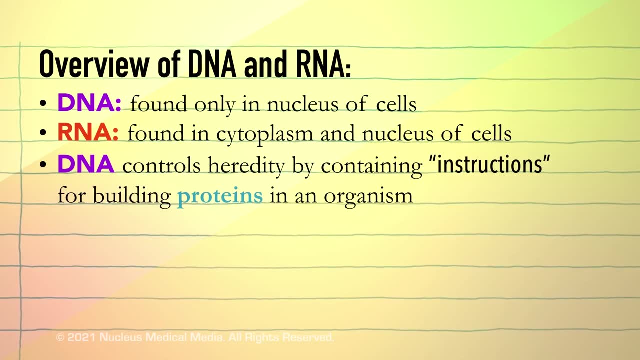 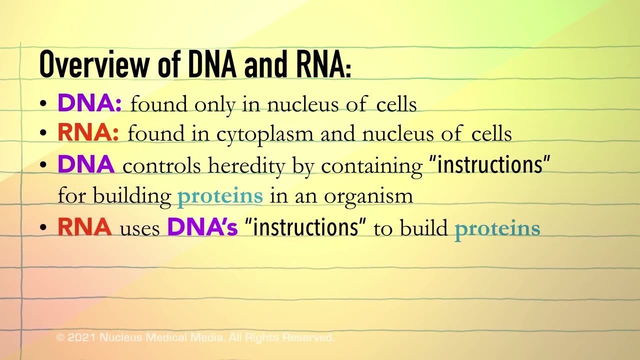 In a cell. DNA is found in the cytoplasm as well as the nucleus. DNA controls heredity by containing the instructions for building the proteins that make up an organism and allow it to function. RNA uses these instructions to build proteins. There are three types of RNA: messenger RNA, ribosomal RNA and transfer RNA.